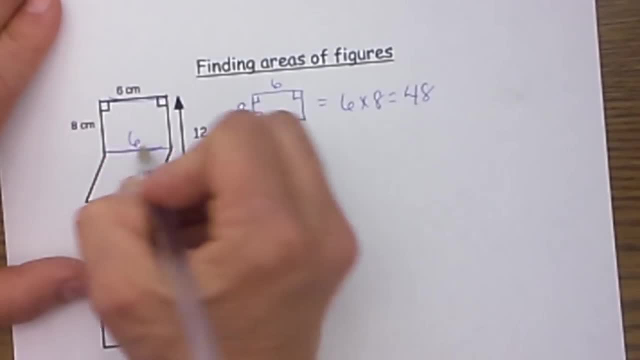 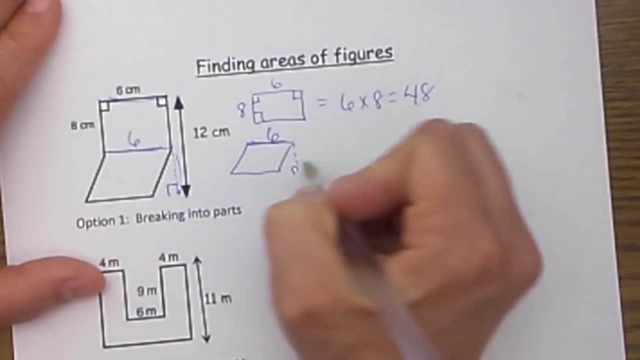 This top dimension is parallel to this top part, so it is also 6.. I will drop an altitude down right here because I need to know this height. The area of a parallelogram is linked to the length times the height, Not the slanted part, but the actual height. I have this. 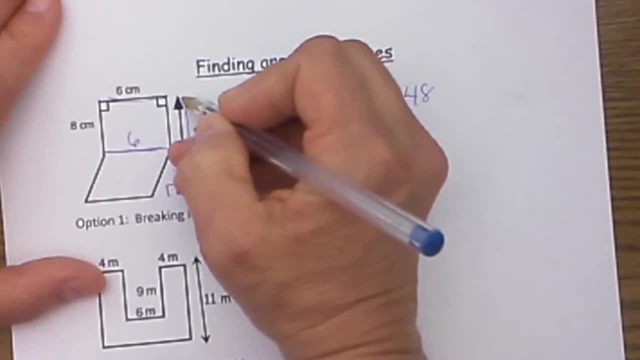 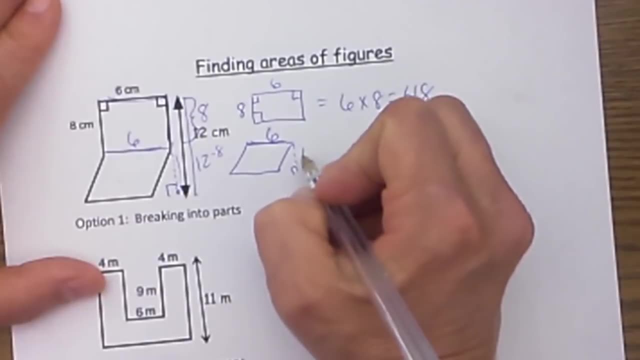 height being 12.. That is the height of the whole figure. What I have to do is take this top portion off, which is 8.. 12 minus 8 is 4.. That is the height or altitude of my parallelogram. 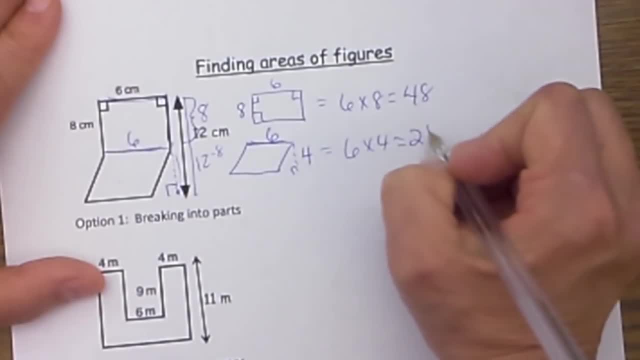 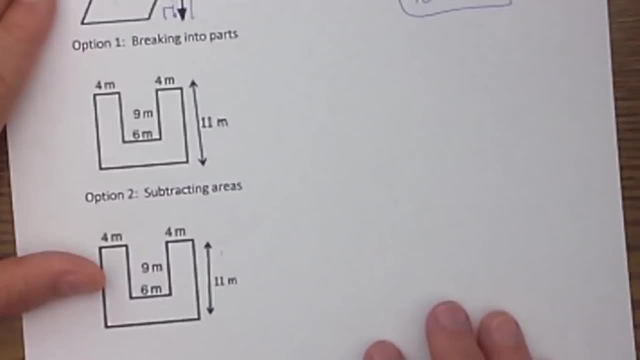 The area of my parallelogram is 6 times 4 or 24, and that adds up to 72 square centimeters. So that is the area of my parallelogram. Now I will take this next figure and we will look at it in two different ways. First, we 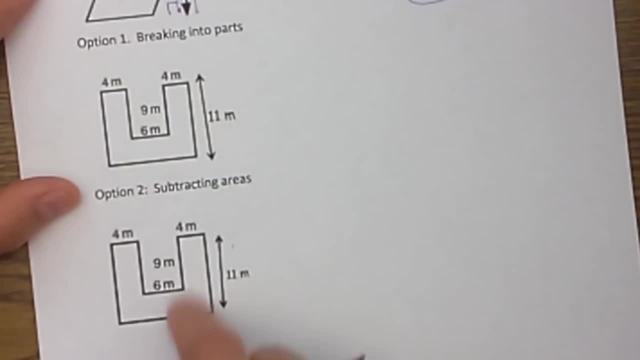 will break it into parts and then I will teach you the subtraction method. This one is just like the top one. I will take this and divide it into parts. I will draw either horizontal or vertical lines to make this line up nicely. I will draw some horizontals. I will draw. 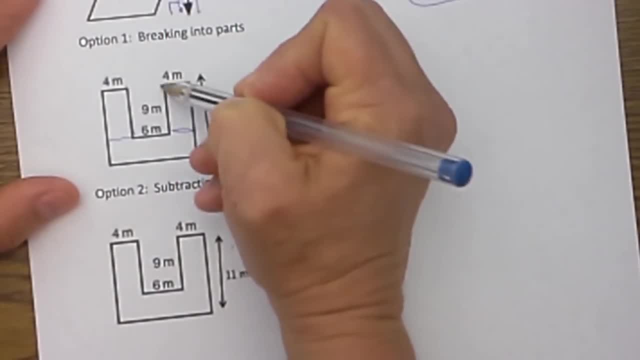 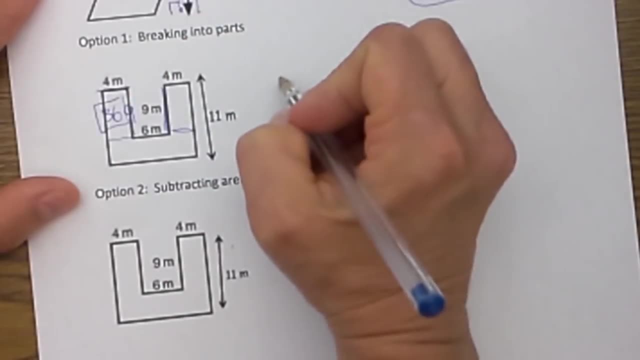 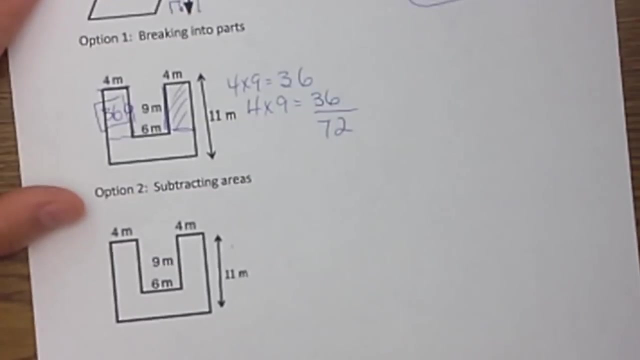 one here and one here. This height here is 9 meters and this length here is 9 centimeters. Length is 4, so that area is 36, because 4 times 9 is 36.. Then I have this other side. that is the exact same, so I will add another 36.. So far I have 72 square meters. 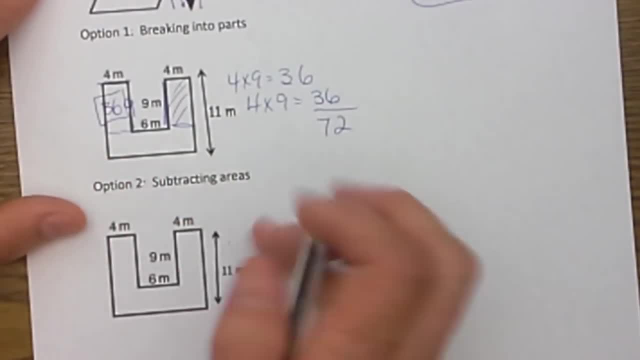 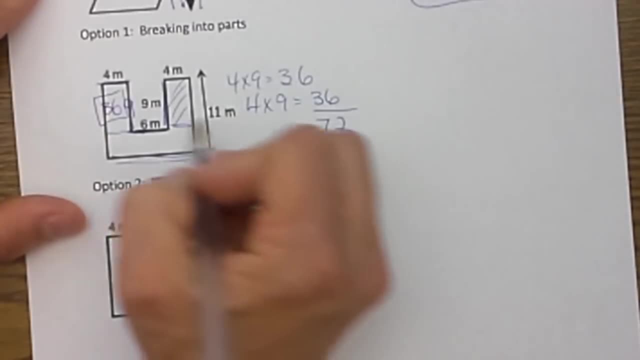 Now let's go down to this bottom section. I know this portion is 6, but I don't have the whole distance across, but I do have the parallel parts. This part we know is 4 and this part we know is 4 because of this top piece. So let's add: 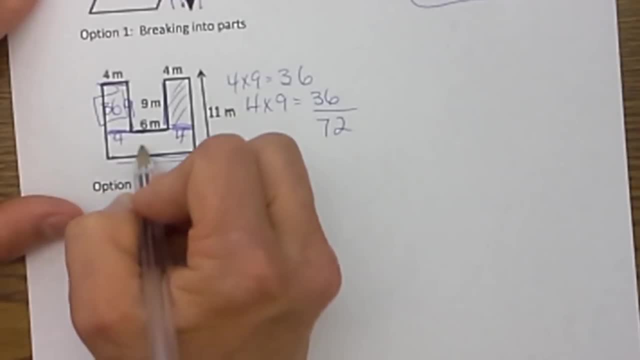 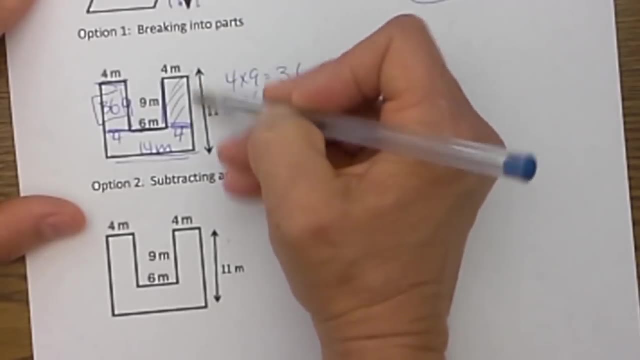 that together, 4 plus 6 plus 4, is 14 meters. Now the height We know, the height of the whole figure is 11.. We have to subtract off the 9 that we know, so this is 2.. So that means 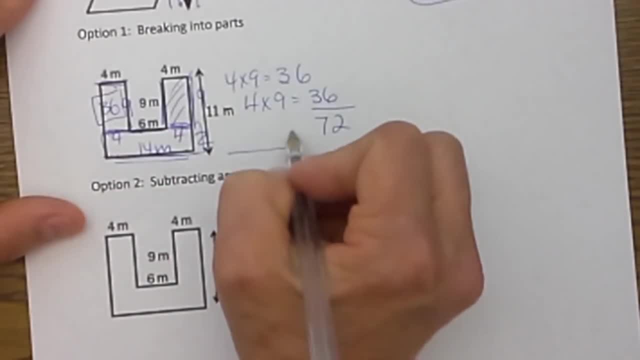 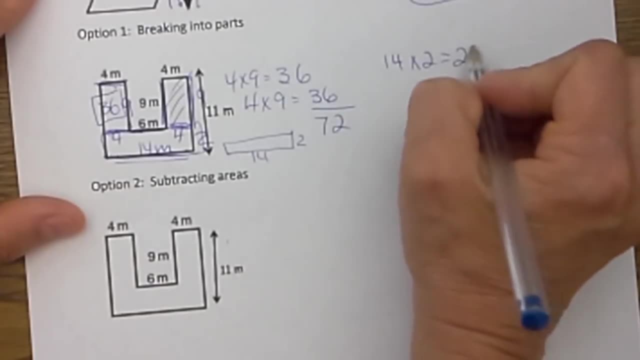 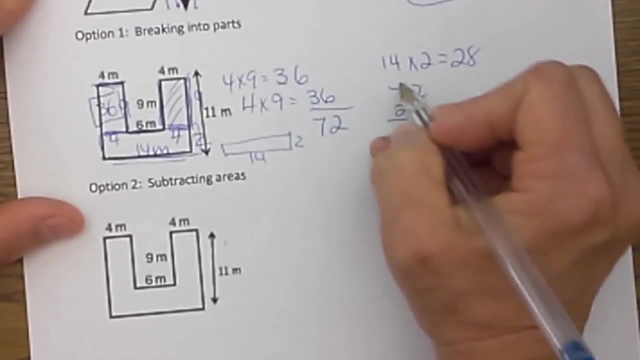 this rectangle down here measures 14.. 14 long, but only too high. So 14 times 2 is 14 meters. 72 gives us another 28 square meters. So let's take 72 and add another 28.. That will give. 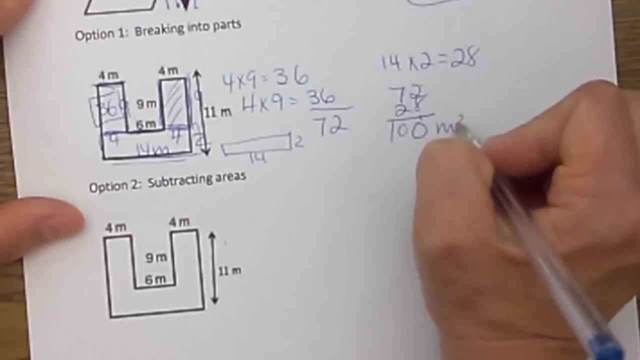 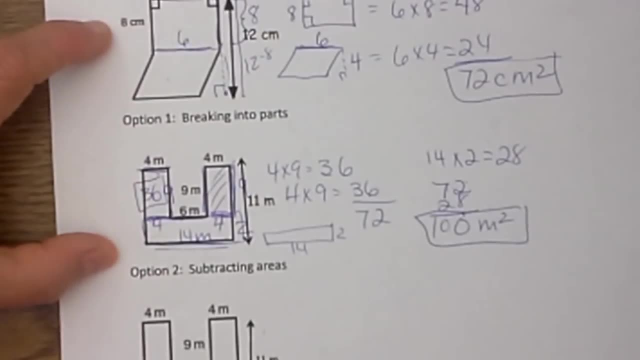 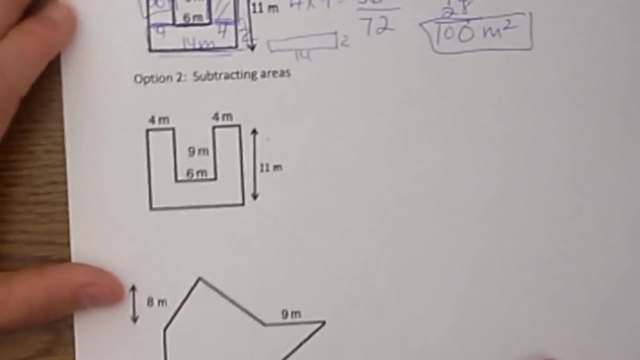 us 100.. 100 square meters for our area. Now that is the way to break it into sections. So that is what the first two represent. Now, this next one is the same figure as the second example. I will show you the subtraction method. What I am going to do is look at it as one. 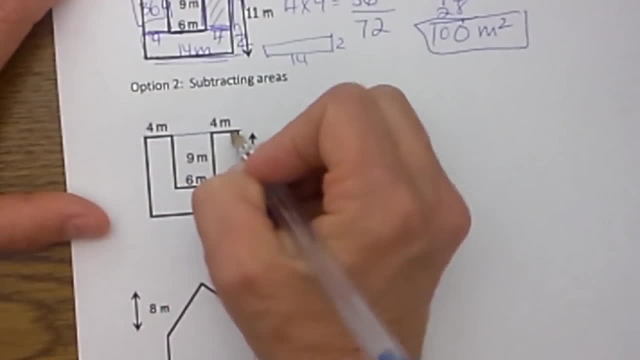 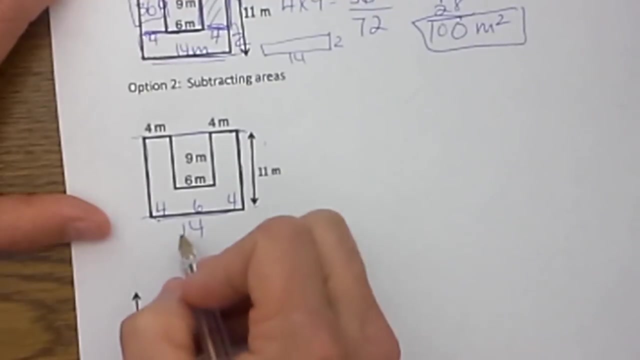 large figure. So I'm going to close this off and I'm going to make a big rectangle So I can now figure out this length. a minute ago we said that was 4 plus 6 plus 4, so this dimension was 14 and the whole side is 11.. 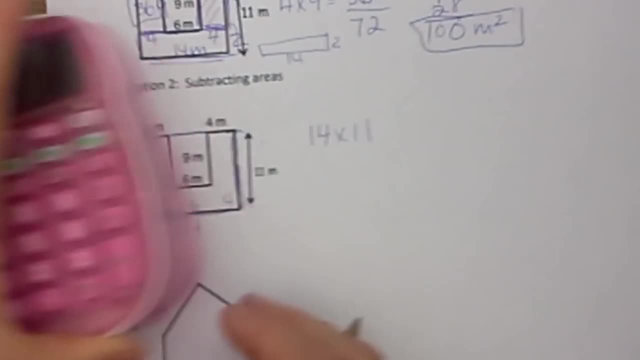 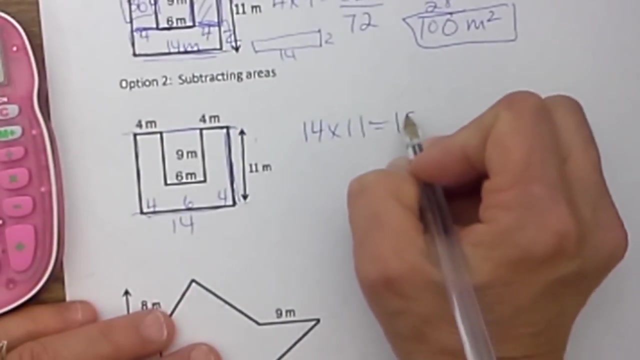 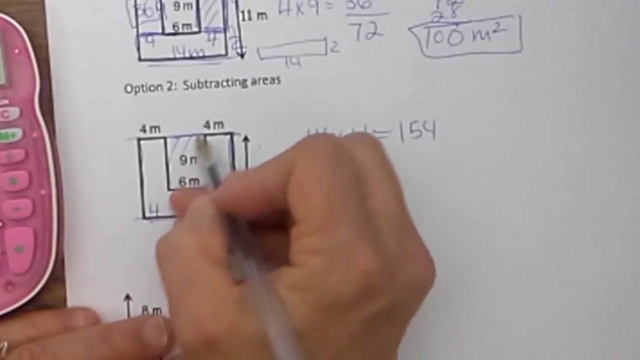 So I'm going to find the area of the entire figure. So let's see, I'm going to grab my calculator for this: 14 times 11 is 154 square meters. Now I need to take out this section that is empty. 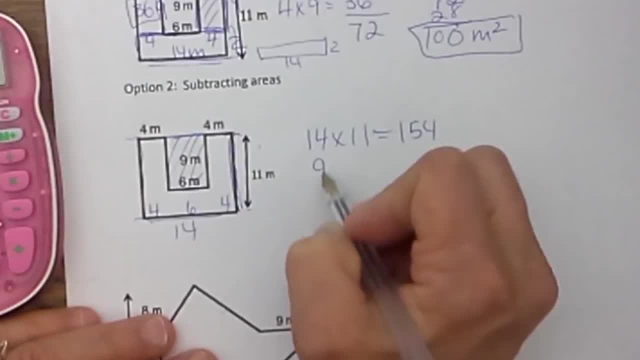 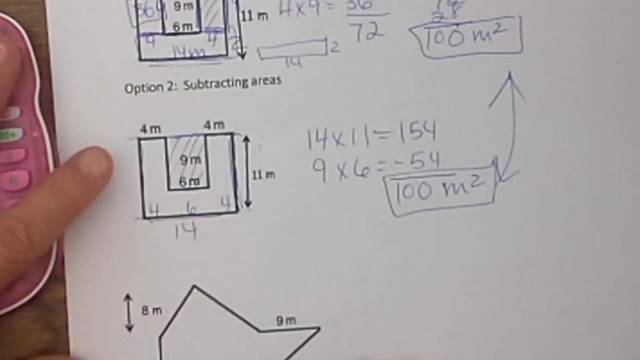 Right here I'm going to subtract off the section that is 9 by 6, 9 times 6 is 54. So when I subtract those two I end up with the same answer of 100 square meters. So those are the two different methods you can use to solve these. 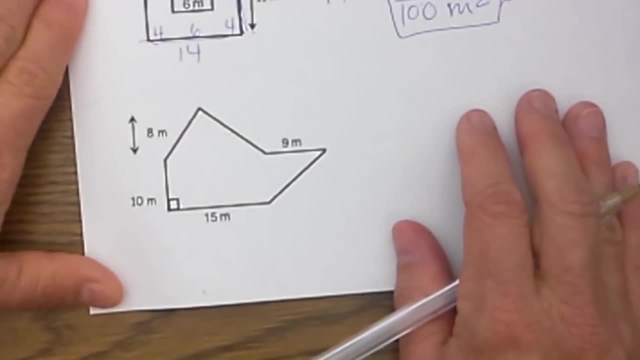 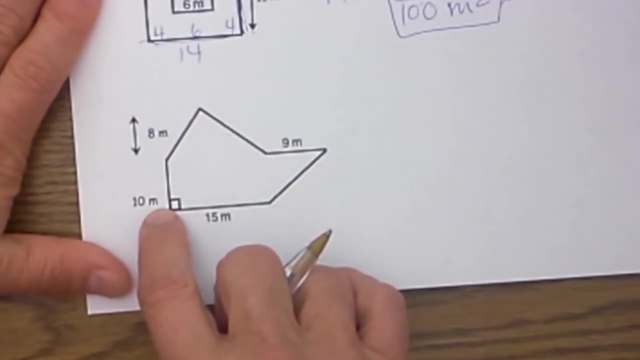 Now let's go down and do one more figure. I wanted to do one that had three parts. This one has three sections, and you could use the method where you fill the whole area in and then subtract parts, but you would have one, two, three parts. 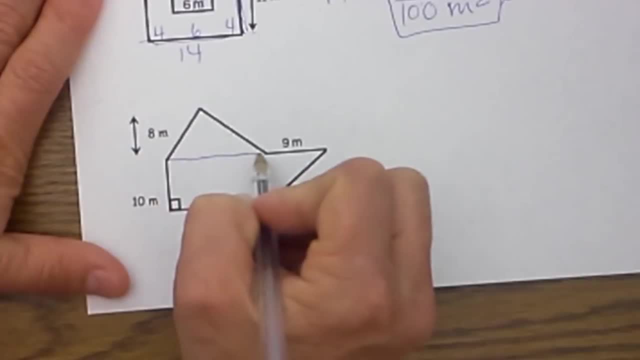 I think this one is just as easy to divide up into sections, So I wanted to do one with a triangle. This one actually has two, So let's see if we can figure this one out. The area of the rectangle is just 10 times 15, which is 150 square meters.